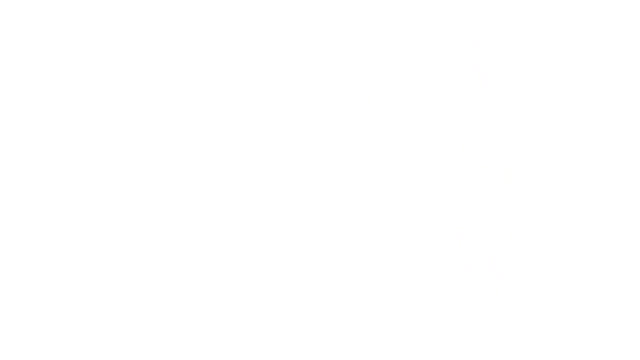 to be focusing on the lower half. Let's start by listing the three types of veins that we can find in the lower limb. The first type of vein we can find are the deep veins, which are usually larger and found deep to the fascia. They are usually paired with arteries, like we see represented here. 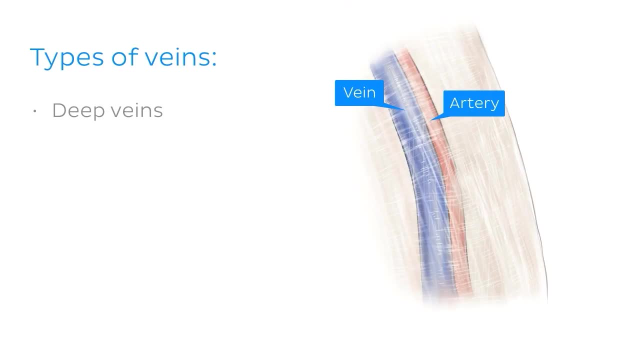 and they're responsible for a majority- around about 85%- of venous return from the lower limbs. The superficial veins are usually smaller and found superficial to the fascia, and you can see an example just here. They're usually unpaired and they're responsible for about 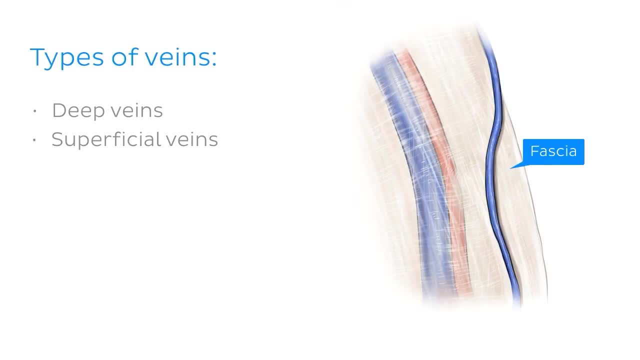 15% of venous return from the lower limbs. Last we have the perforating veins, which connect the deep and superficial veins and run to the fascia which is shown in the image. Now let's get into some more specific anatomy, starting with the deep veins. 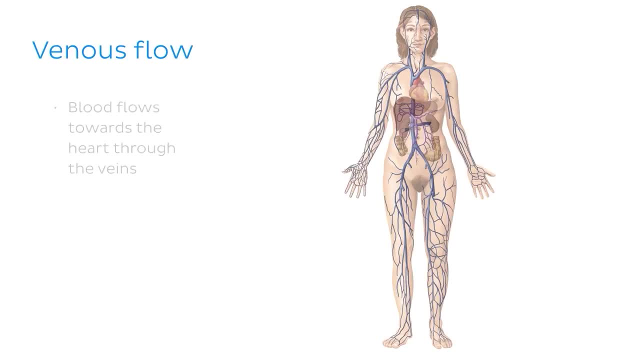 So we're going to begin at the bottom of the foot and remember, blood flows towards the heart through the veins, So in the case of the lower limbs it's always going to be from the feet up, so we're starting at the beginning, in a way. 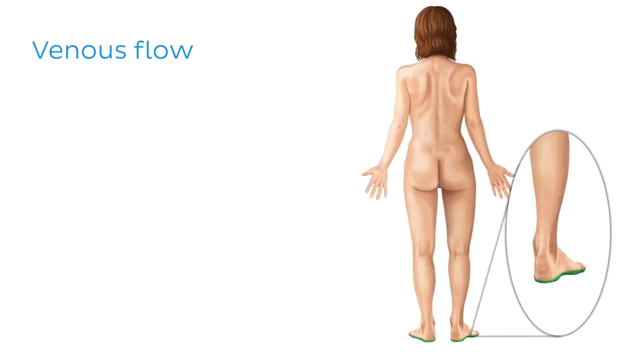 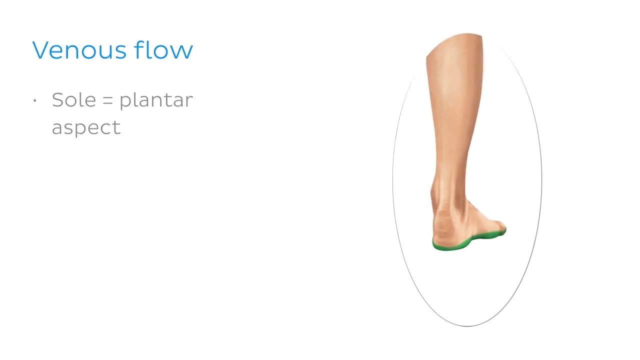 And the aspect of the foot that we're going to be looking at is also called the plantar aspect, which you can see in this image, And just note that the images we'll be looking at will mainly be the right foot. so this side will be our medial side and this side will be our 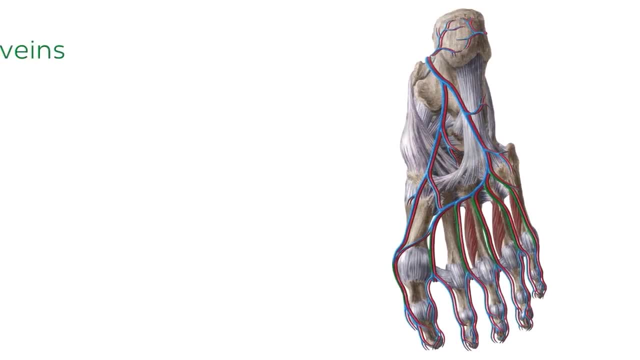 lateral side. So in this image we can see the plantar metatarsal veins and arteries which are on the sole of the foot, And the plantar metatarsal veins run along with the arteries here which you can see in red. The plantar metatarsal veins arise from the plantar digital veins of the toes and communicate. 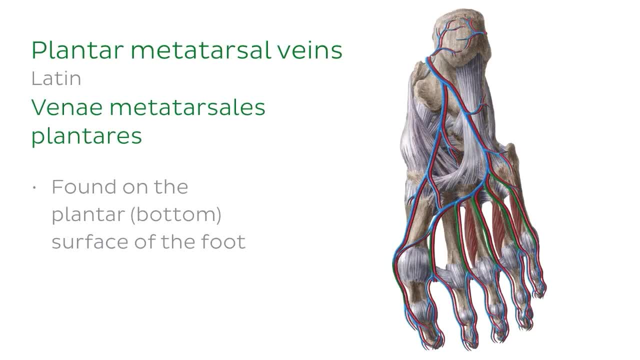 with the veins of the dorsum or the top of the foot. The plantar metatarsal veins run medially within the intermetatarsal spaces which you can see outlined in blue in this image, And they're also running medial to the artery. 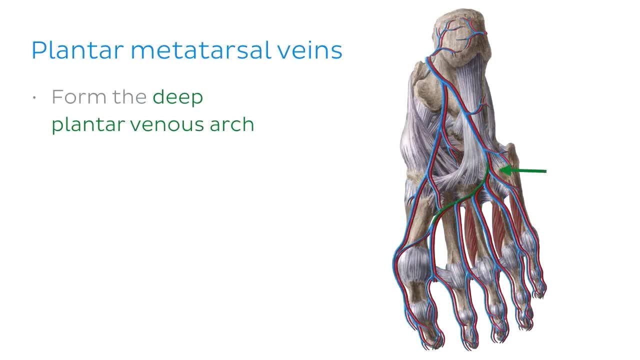 The veins then continue onwards to form the deep plantar venous arch which we see here, And note that the medial and lateral plantar veins arise from this arch. So let's continue to the veins found on the dorsal or the top surface of the foot.